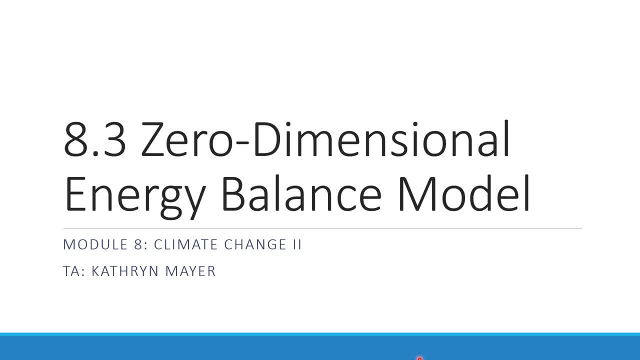 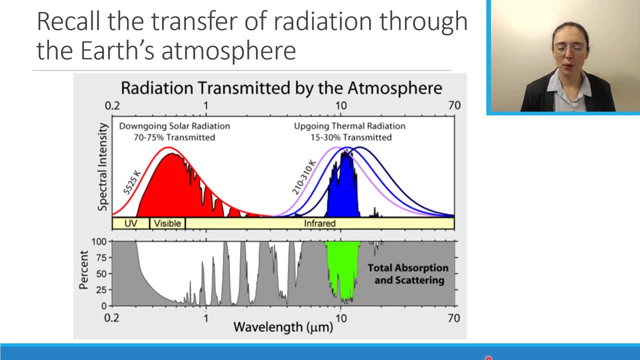 going to see if we can use these very simple equations to predict the temperature of the Earth's surface. So, to start, I want you to recall the transfer of radiation through the Earth's atmosphere. I know we've gone over this a hundred times, but just as a reminder there's incoming 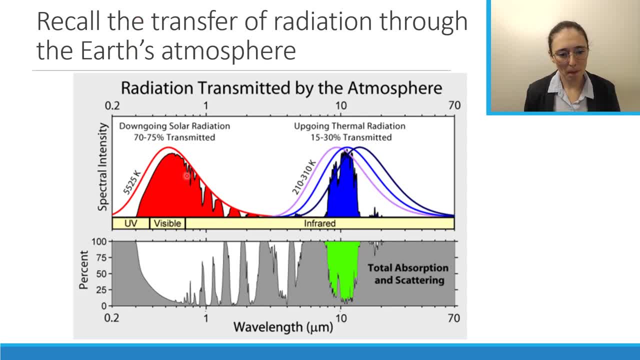 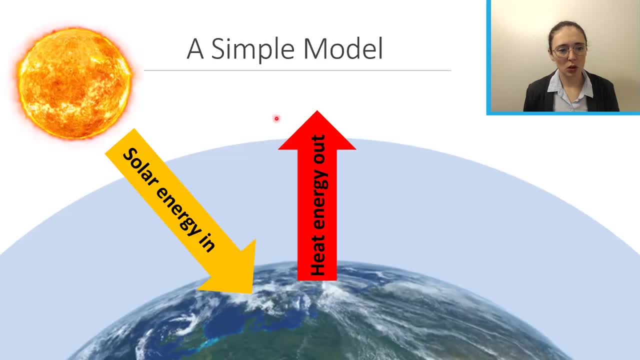 solar radiation from the Sun that's in the UV visible region, that gets absorbed by the Earth's surface and then re-emitted as up going thermal radiation. So this is what this looks like: You have solar energy in and then heat energy out from the Earth. Now, if we add a little bit more, 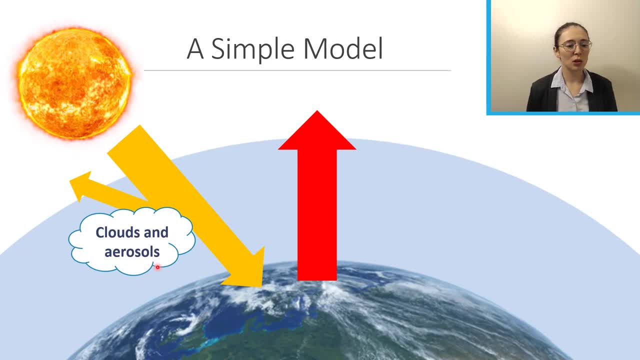 complexity. clouds and aerosols reflect some of this incoming solar radiation, so not all of it reaches the Earth's surface and gets absorbed. We also have greenhouse gases which are going to trap some of this heat and warm the Earth's surface, because the energy can't escape out into space. 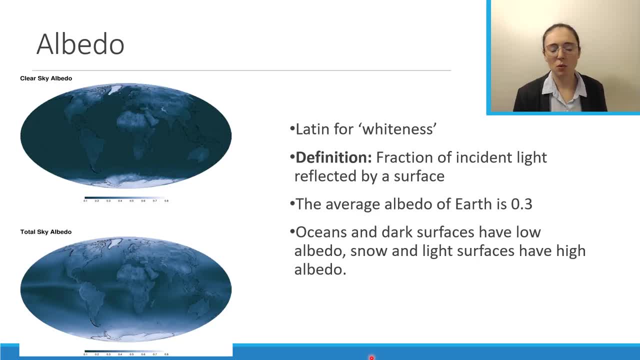 Okay, so we've talked about albedo before, but I just wanted to find it formally before we move on. It is literally Latin for whiteness, and the definition is the fraction of incident light reflected by a surface. So you know this intuitively right: Dark objects are going to. 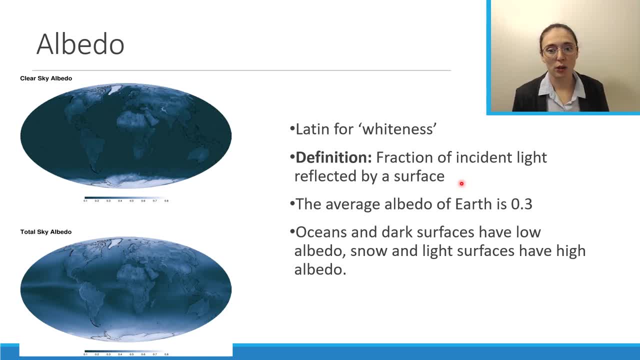 absorb more solar light. more sunlight, Light colored objects are going to reflect more, right, If it's a really hot day, it's bright, sunny. you probably don't want to choose a black shirt. Wearing a white shirt might make you cooler. This is something you just know intuitively from your 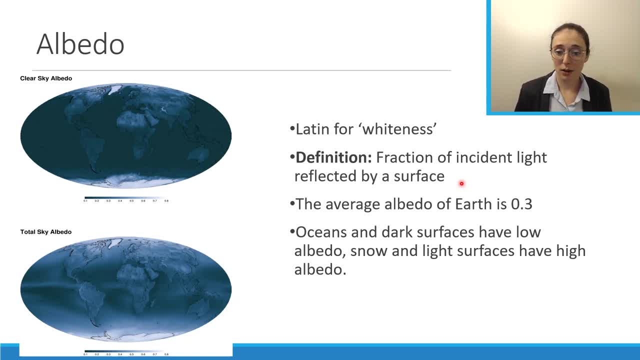 experiences in the world. So this is true for the Earth as well. The average albedo of the Earth is about 0.3.. So that means that about 30 percent of the incident light from the sun is actually reflected just back out into space. So oceans, other dark surfaces have low albedo, whereas snow and light 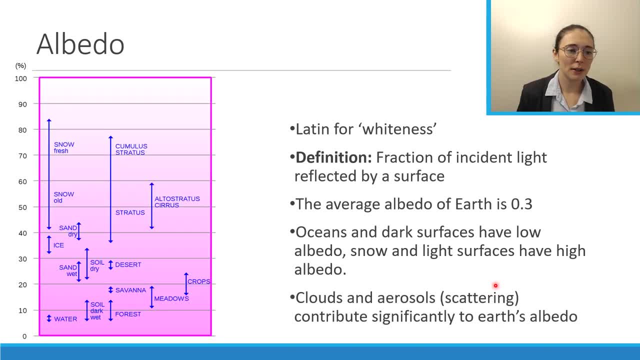 surfaces like ice have high albedo. We also have a significant amount of our atmosphere's albedo comes from clouds, which scatter, and also aerosols, which scatter and reflect light. So this is a figure showing the fraction of light reflected for different surfaces. So we see that. 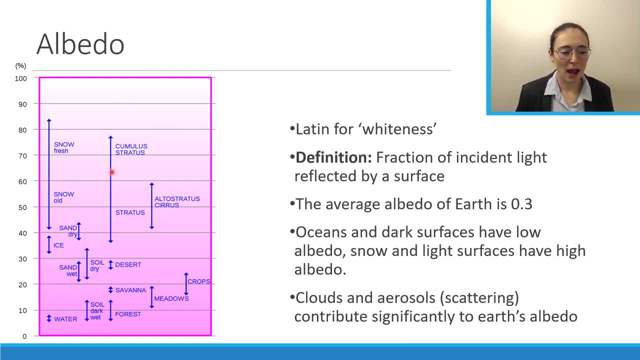 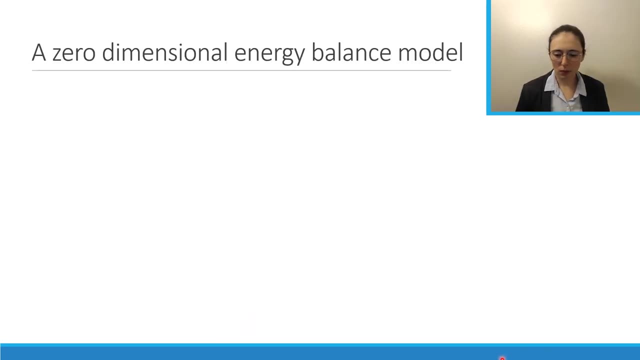 snow is very high. ice, different types of clouds, even desert and sand are somewhat high. and then we see for our darker surfaces, like forests, soil, water, etc. those have lower albedo, they're going to absorb more light. Okay, so let's move on to our zero dimensional energy balance model. So, to start, 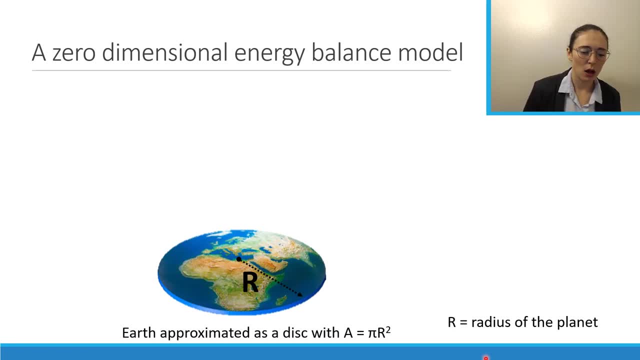 flat disk with a radius R, and so this is going to have an area of pi R squared. Now, the reason we're approximating the earth as a disk instead of as a sphere is because, when it's daytime, solar light is going to be hitting half of the 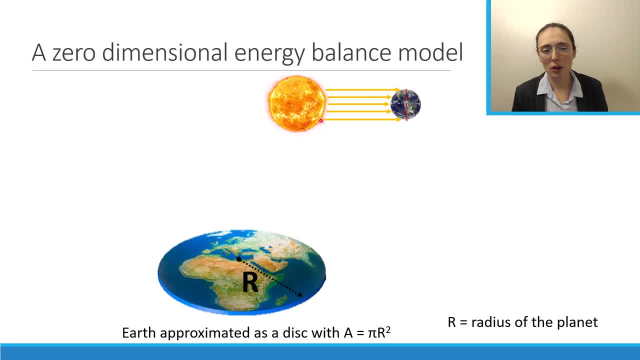 planet, and instead of accounting for differences in solar insulation with latitude, we're just gonna say that the same amount of light hits this half of the planet when it's daytime. So this really simplifies our model. we just have a disk earth to worry about, and all parts of the disk earth get the same. 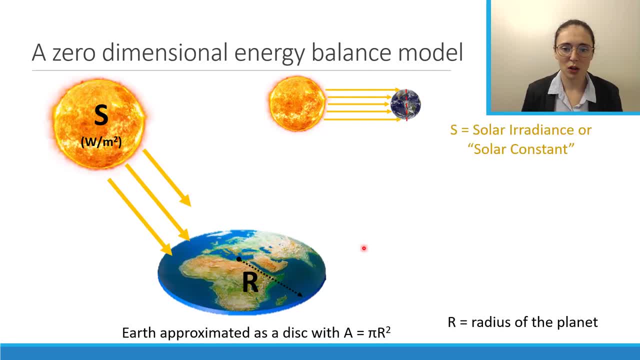 amount of solar radiation. Now the next part of our model is going to be the Sun, So the Sun shines on the earth and the amount of light in watts per meter squared is going to be the solar radiance s or the solar constant. Then we 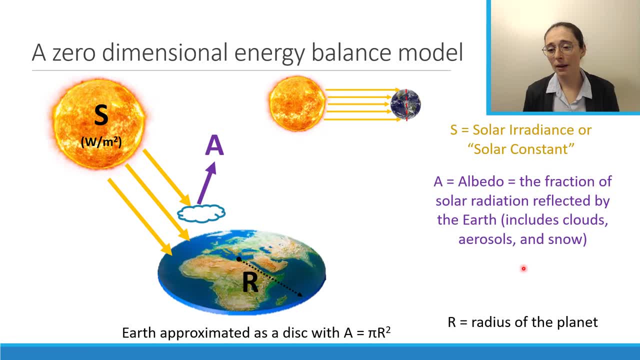 have our R squared. R squared equals Albedo, so that's going to be the fraction of light that is reflected from the earth, So that's going to be a. and then we have F, which is the flux of long-wave energy emitted by the planet. 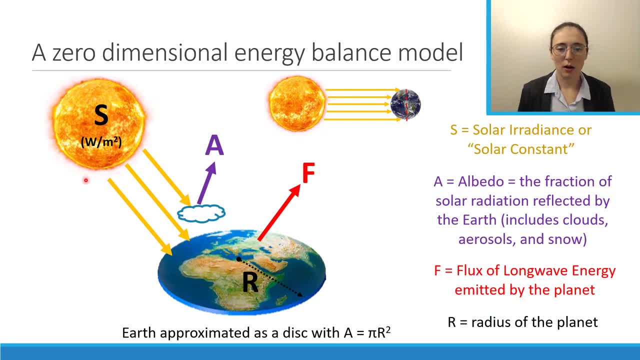 This is the start of our energy balance model. these are our four factors that we need to account for: the radius of the earth, The solar insulation, the solar radiants, The fraction of light reflected and then the flux of outgoing long wave wave. So in our zero-dimensional energy balance model, the solar energy incident. 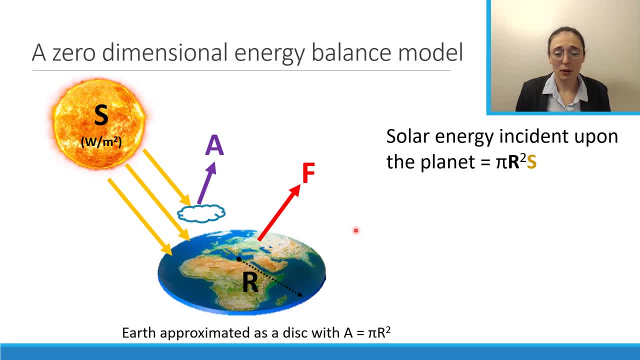 upon the planet is equal to pi r squared s. So that's the area of the Earth's surface times the solar irradiance. Notice: here the units of s are in watts per meter squared. so if we multiply s by the area we'll get a answer out in watts. 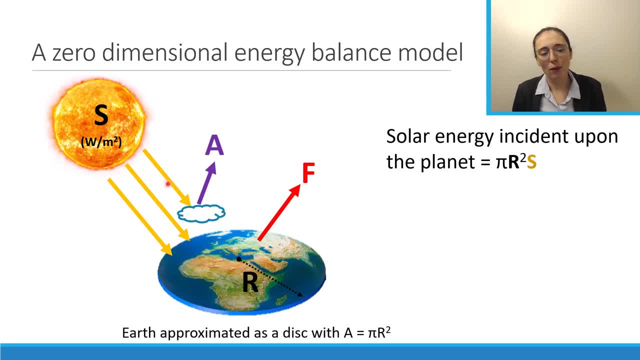 which is what we want. Now we need to account for the albedo, since some fraction of that incident light is reflected, so the solar energy that actually makes it to the Earth's surface is going to be equal to pi r squared s times 1 minus the albedo. So that's because, whatever the albedo is for our 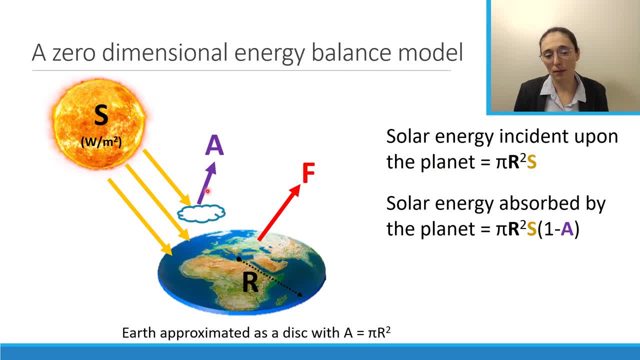 case it's about 0.3 or 30%. about 30% of that light is reflected. it never makes it to the surface. So that's because, whatever the albedo is- for our case it's about 0.3 or 30%- about 30% of that light is reflected. it never makes it to the 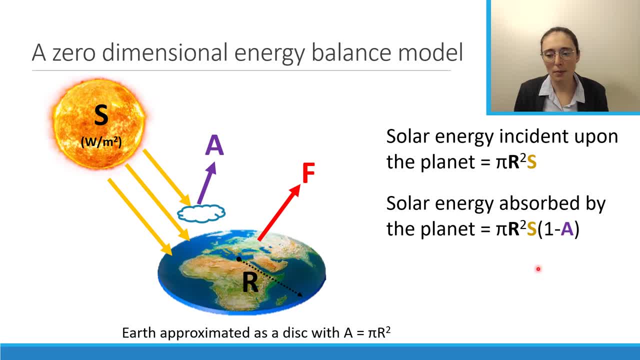 surface. So we'll just multiply the incident light times 1 minus the albedo, and that gives us the energy that actually is absorbed by the planet. Finally, the energy emitted by the planet is going to be equal to 4 pi r squared f, where f is the flux of outgoing long wave. Okay, so for an energy balance. 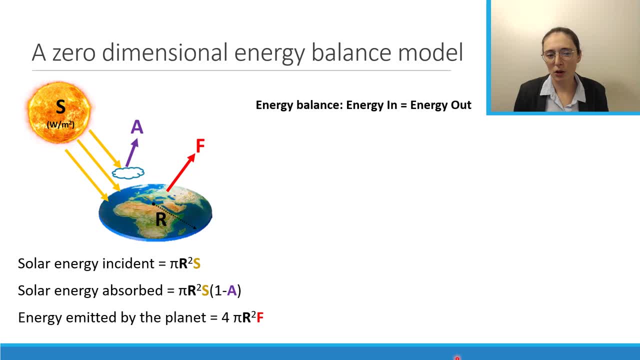 model. we need energy in to equal energy out. So that means that we're going to set our incoming solar radiation equal to our outgoing terrestrial radiation. So we have pi r squared s. 1 minus albedo equals 4 pi r squared f. So we've set our solar incoming radiation equal to the. 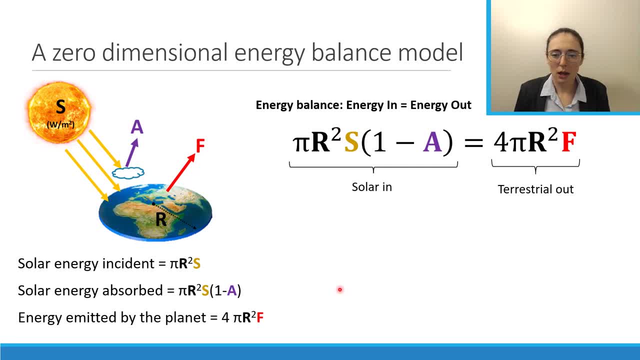 outgoing terrestrial radiation. Now we need to solve for f, so we're going to approximate. the Earth has a black body, so we'll use the Stefan Boltzmann law where f is equal to Sigma times TE to the flesh point into加 to g, That's called the. 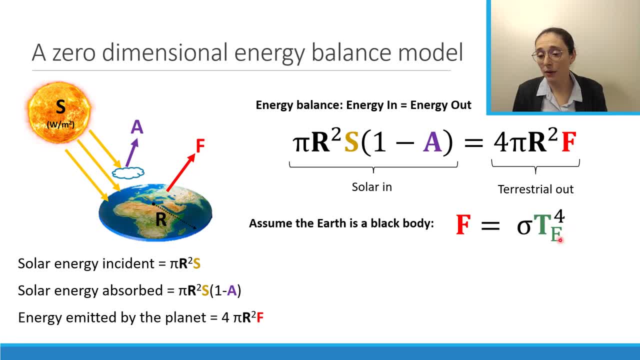 fourth, where Te is the effective temperature of the earth's surface and sigma is the Boltzmann constant. So if we plug this in, we get our global energy balance equation, which is pi r squared s one minus the albedo, equals four pi r squared sigma times Te. to the fourth power. Now we can. 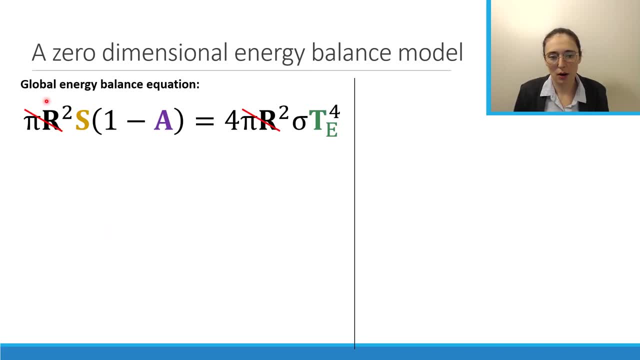 obviously simplify this equation a bit. so if we cancel out our pi r squareds and rearrange this and solve for the effective temperature of the earth's surface, we get this relationship. Te effective equals the fourth root of the solar irradiance times one minus albedo over four times. 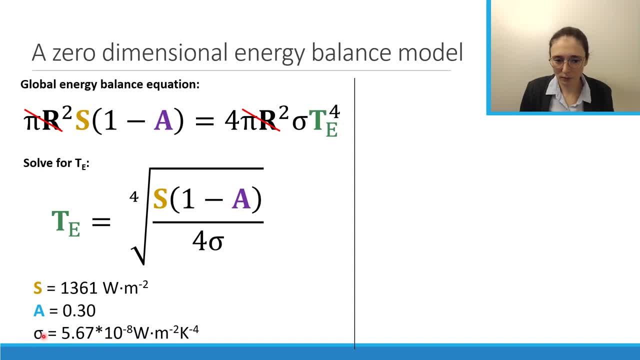 sigma, where sigma is the Boltzmann constant. Now, as we discussed before, the albedo of the earth is about 0.3 and the solar irradiance is approximately 1361 watts per meter squared. Now this actually varies on a decadal scale, but this is the number we can use for right now. So 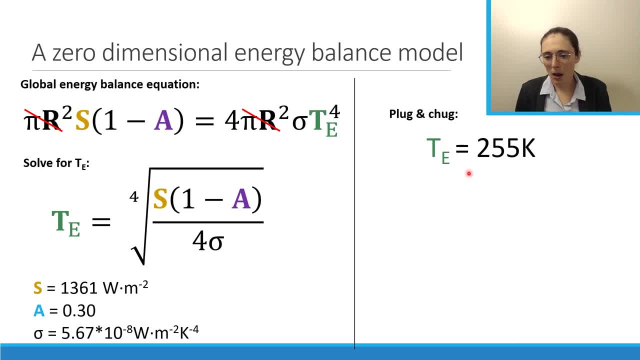 if we plug all these numbers into the equation, well, you'll get 255 Kelvin. If you don't believe me, you can go solve this math by just plugging in these numbers into the equation. So you get the temperature of the earth's surface and the observed surface temperature. Now, the observed 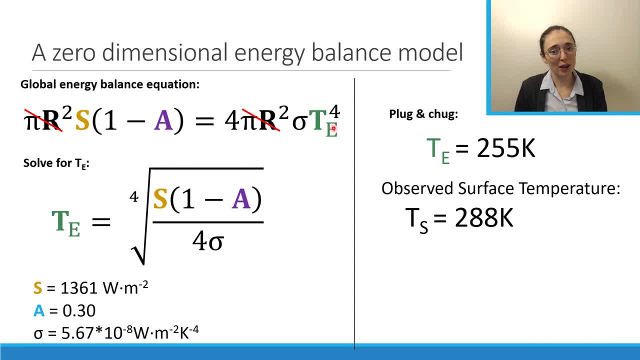 temperature of the earth's surface is 288 Kelvin. So we have a 33 degree Celsius difference between our model that we're getting from our energy balance model and the actual observed surface temperature of the earth. So why is the observed temperature higher than the calculated temperature? 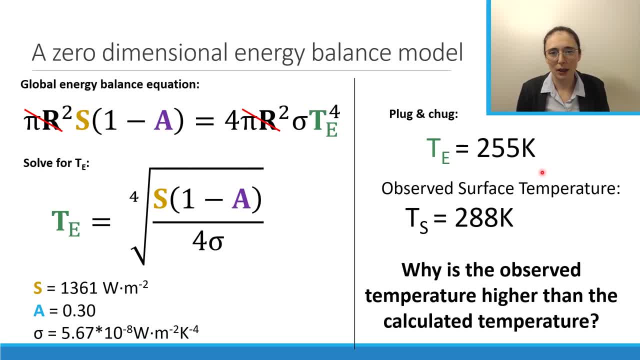 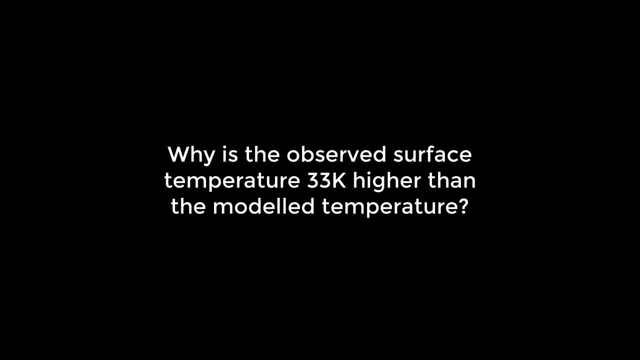 I'll just give you a second to think about that before I move on. Why is the observed temperature higher than the calculated surface temperature temperature from the model? OK, so I hope you were able to guess it, The reason our observed temperature is so much higher. 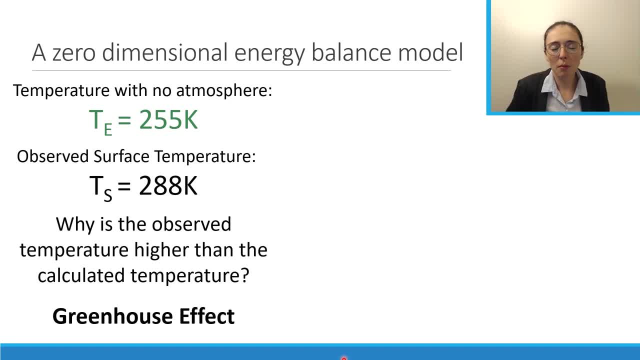 than the calculated temperature is because of the greenhouse effect. Our model doesn't account for the absorption of outgoing long wave by the atmosphere, So that 33 degree difference between our calculated surface temperature and our observed surface temperature is really driven by the greenhouse effect. 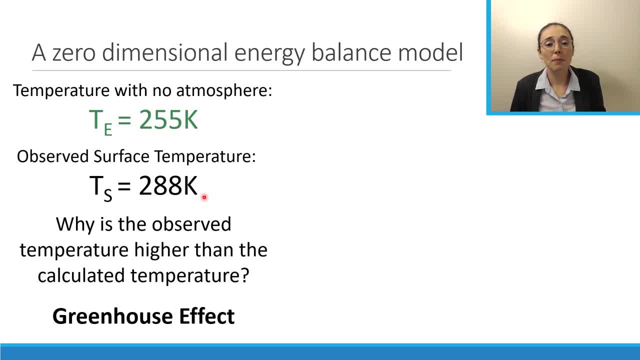 I'm not talking about the anthropogenic greenhouse effect during amplified greenhouse effect during the 20th and 21st century. What I'm talking about is the natural greenhouse effect, So that's the water vapor and carbon dioxide that are naturally in our atmosphere. 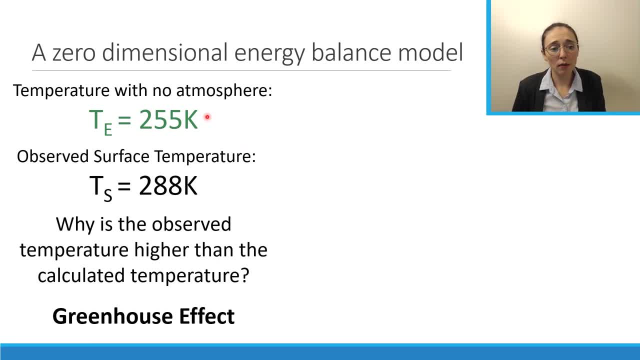 that warm the atmosphere from 255 Kelvin to 288,, which is a much warmer and more habitable temperature for the life that at least currently inhabits Earth. So how can we fix the model? Well, we can do that by adding a tuning knob to get this right. 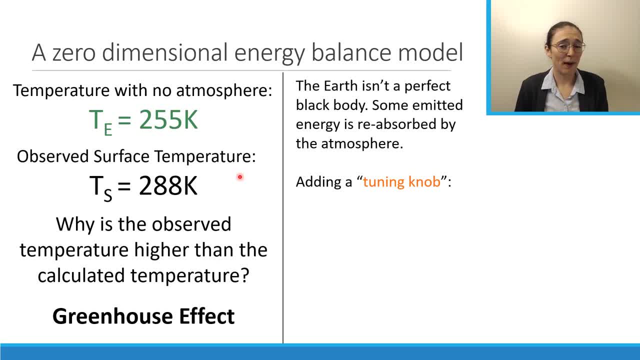 So an easy way would be to add a tuning knob. Essentially, we can add a fudge factor that accounts for some of this reabsorption of energy in the atmosphere. So what this looks like is that we'll add an emissivity factor, E or epsilon. 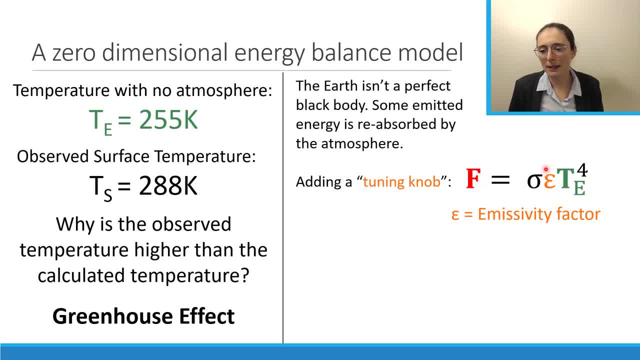 to the Boltzmann equation. So F equals sigma times epsilon times Te to the fourth power. So what we get is that the effective temperature equals the fourth root of s times 1 minus a times 4 epsilon sigma, where we have our emissivity factor plugged. 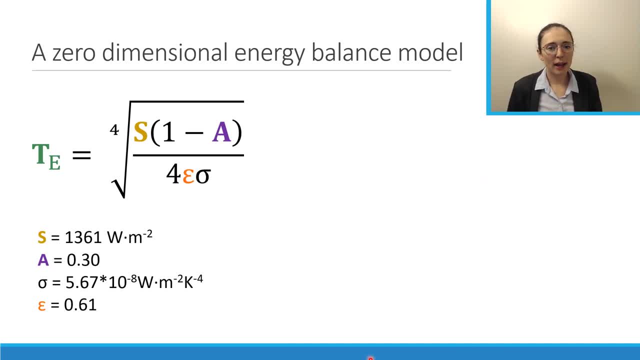 in here. So if I plug in 288 Kelvin for Te and I solve this out, I'll get a value of epsilon that's approximately 0.61.. And so what we can do is essentially plug this into our model, and it makes it work. 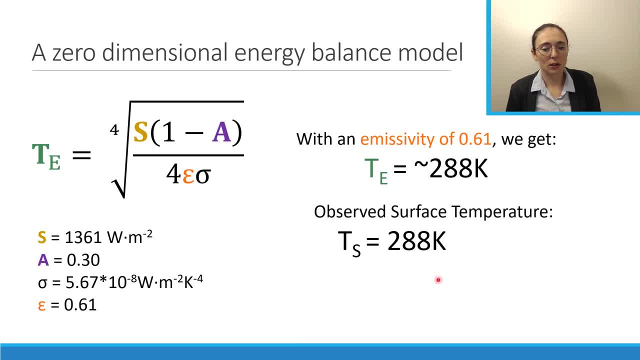 So we're able to calculate an effective temperature that's equal to the surface temperature. So this is a really simple model and it's a bit fudged, But we can actually still use this equation to look at how the climate system might react to changes. 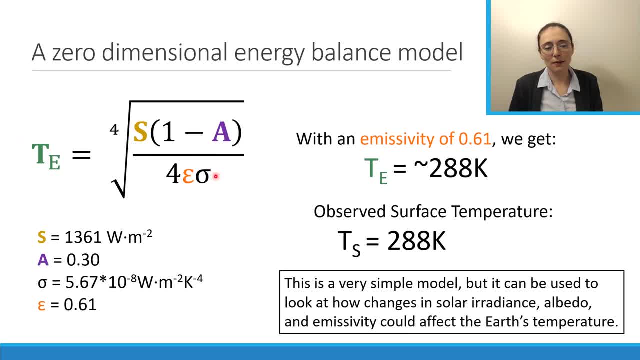 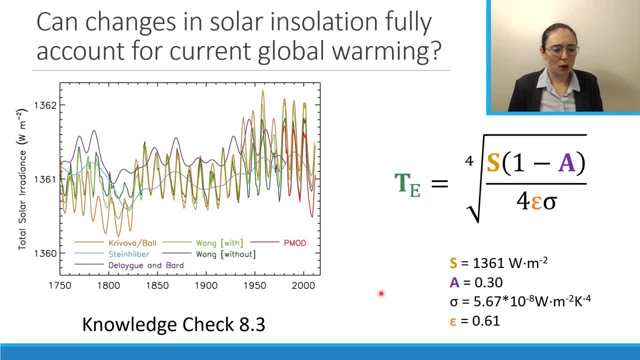 in solar irradiance, albedo or even the sensitivity to the emissivity factor of the atmosphere. OK, So a question I have for you guys is: can changes in solar insulation fully account for current global warming? So this is a plot from the IPCC Fifth Assessment Report. 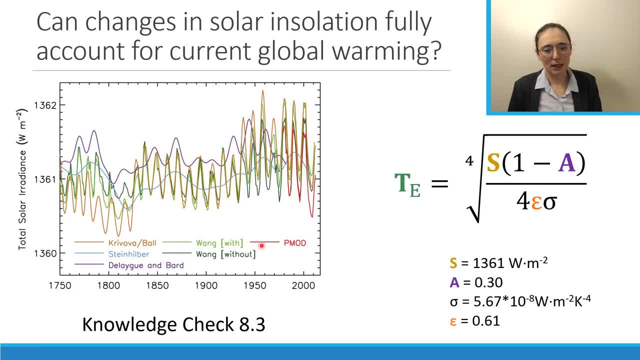 that shows changes in solar insulation since 1750. So we can see that there is- I think it's- an 11-year cycle that solar irradiance goes through And while there's a bit of disagreement between some of the past reconstructions, 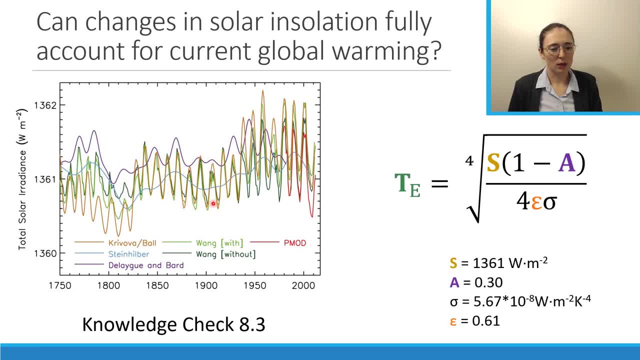 of the solar irradiance. we can see this clear trend where the solar irradiance goes up and down on a cycle, And so this is something that gets brought up a lot with climate skepticism is: can't we just explain climate change with solar irradiance? 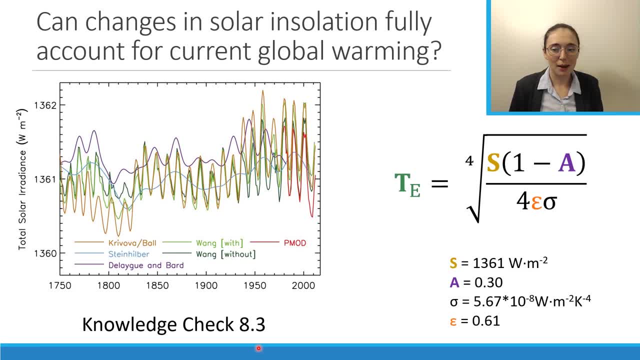 So what I want you guys to do is for knowledge check 8.3,. you're going to use this equation with these constants to calculate how much the Earth's temperature would change due to shifts in the solar irradiance. So you should see knowledge check 8.3.. 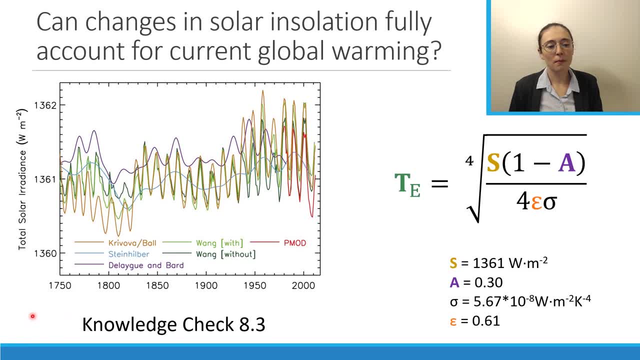 OK, Let's check 8.3 for more instructions on that, But this is the equation here that you'll be using to calculate how much temperature might change with solar irradiance, And so this is a really good use of our simple model, because we should actually be able to capture. 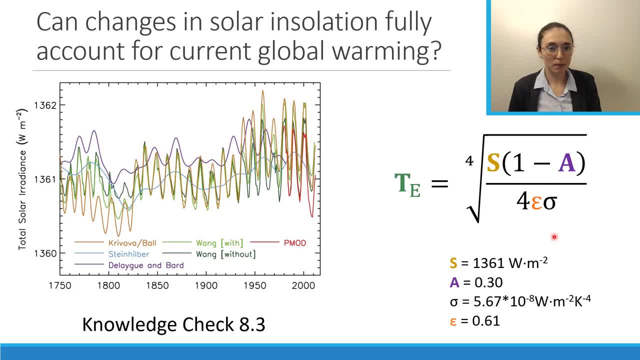 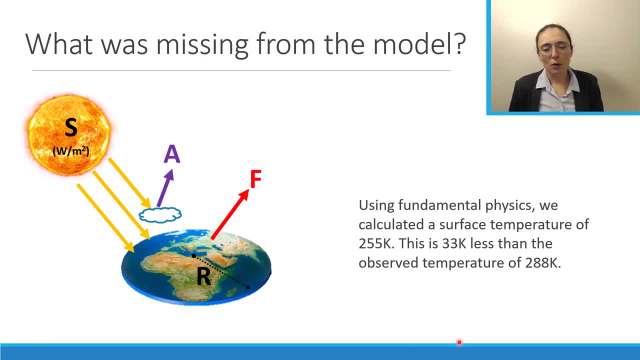 this effect to some degree of accuracy with this very simple equation. All right, So now let's think about what was missing from our model. Using fundamental physics and the stuff in Boltzmann, we calculated a temperature that was 33 Kelvin less than the observed temperature of 288 degrees Kelvin. 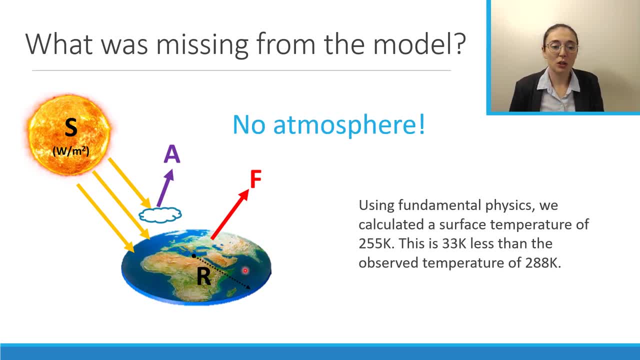 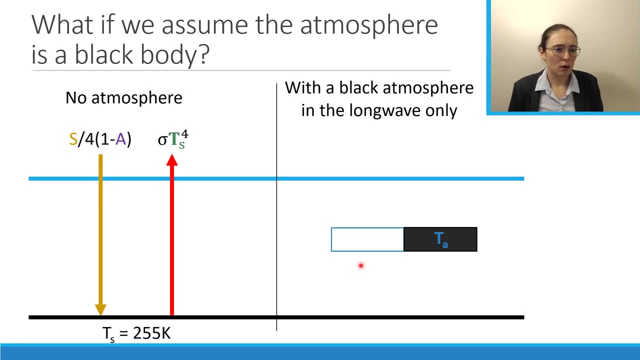 So the problem was that we don't have an atmosphere in our model. There's literally nothing here that represents the atmosphere. That emissivity factor was just a fudge factor on the outgoing long wave flux, So how could we include an atmosphere in this simple model? 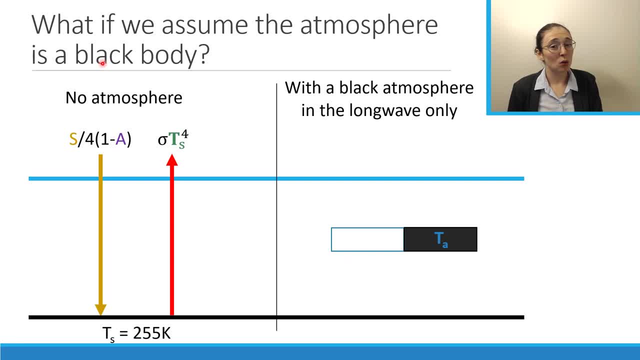 OK. So what would happen If we assumed that the atmosphere emitted as a black body? So with no atmosphere, we just have solar radiation in, And then we have long wave going out. So this is all we had in our original zero-dimensional model. 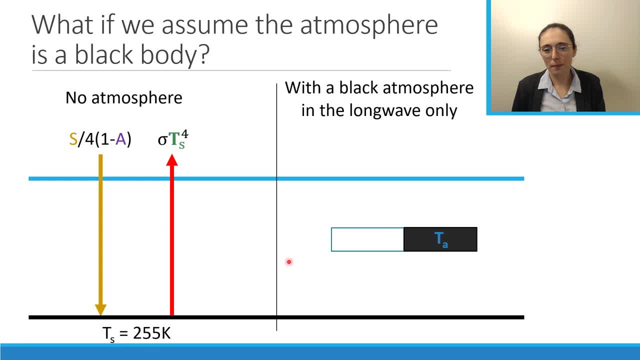 And we got a surface temperature of 255 Kelvin. Now with a black atmosphere. so that's an atmosphere that's going to emit as a perfect black body in long wave. only what do we get? So we still have solar coming in. 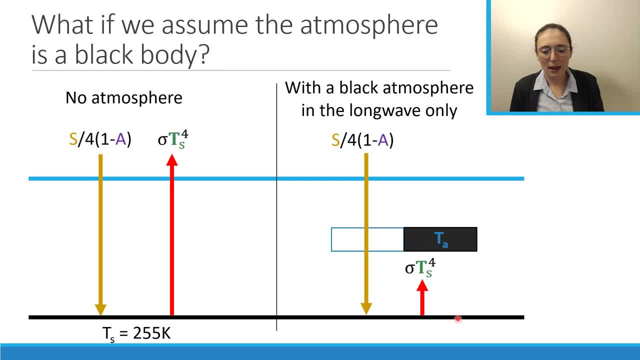 So solar light comes in, It is absorbed by the surface And then it's re-emitted. So we still have this sigma Ts, where Ts is the surface temperature to the fourth power is our outgoing flux, And then that gets absorbed by the black atmosphere. 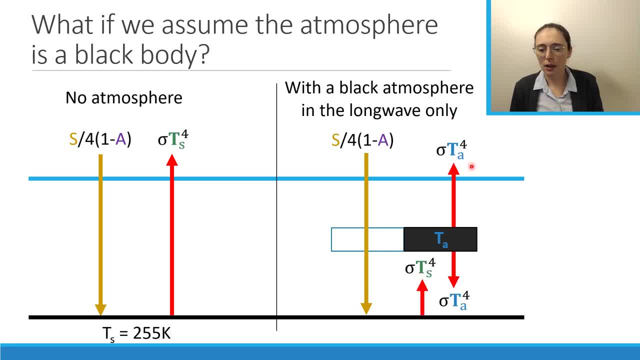 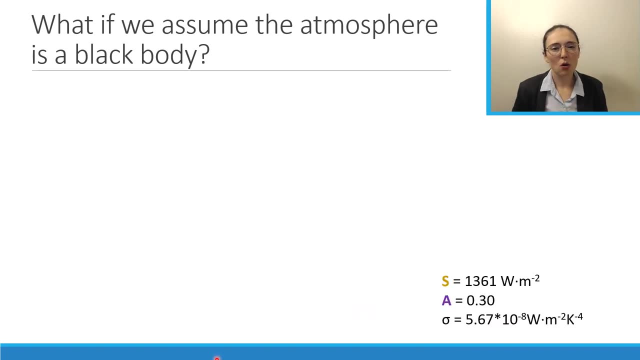 and re-emitted in both directions, except it's going to emit at the temperature of the atmosphere. So here we have sigma Ta to the fourth. We also have sigma Ta to the fourth going downward. OK, so now, assuming that the atmosphere absorbs and emits, 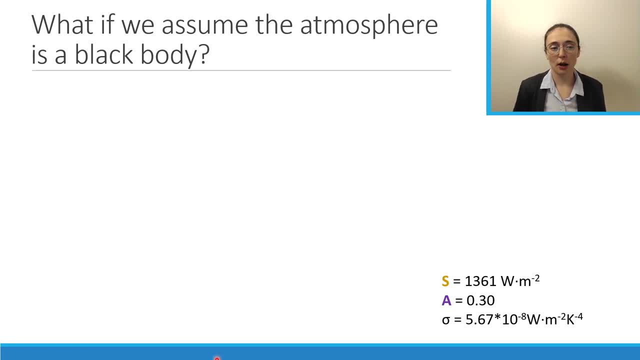 as a perfect black body. let's calculate the surface temperature of the Earth. So to start to have energy balance at the top of the atmosphere, the incoming solar radiation has to be equal to the outgoing long wave emitted by the atmosphere. And to make things simpler for ourself, 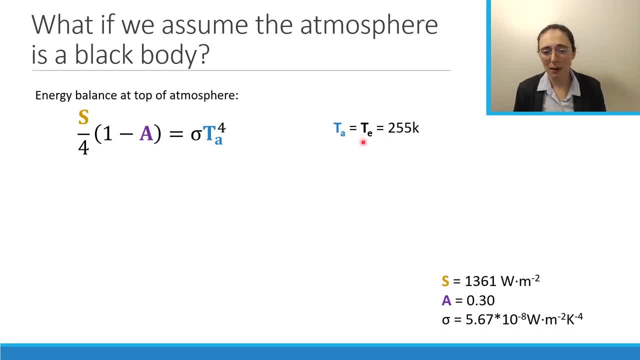 we're going to set Ta- the temperature of the atmosphere- equal to the Earth's effect Effective temperature, which is 255 Kelvin. Now we also have energy balance at the surface, So here we need to set the long wave flux. 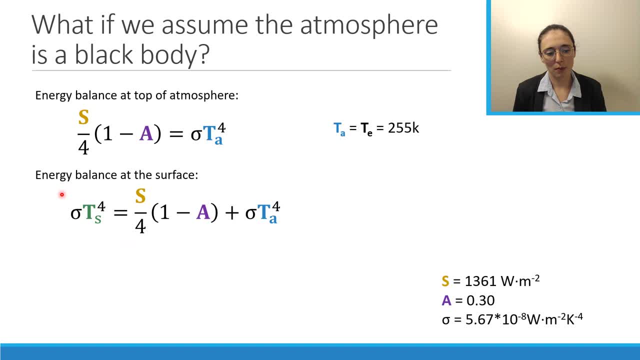 from the Earth's surface. So that's going to be Ts to the fourth power times sigma, equal to the incoming solar radiation plus the long wave flux emitted from the atmosphere. So remember, the atmosphere is emitting black body radiation in both directions: It's emitting it up and it's emitting it back down. 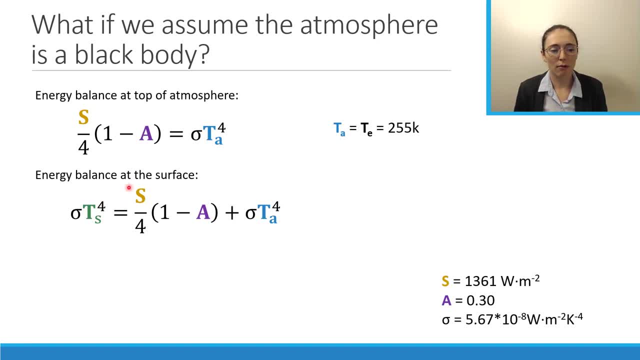 towards the surface. So we have at the surface we have both the incoming solar light as well as the long wave flux that's actually emitted back downwards by the atmosphere. Now we're going to solve this for Ts. So what we get is the fourth root of S times 1 minus A. 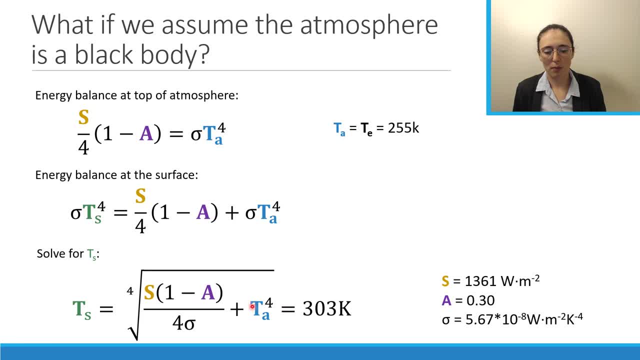 over 4 sigma plus Ta to the fourth power. And if we solve this all out using 255 Kelvin in our constants from before, we get 303 Kelvin Now, T surface being 303 Kelvin is much warmer than the observed surface temperature, which is 288 Kelvin. 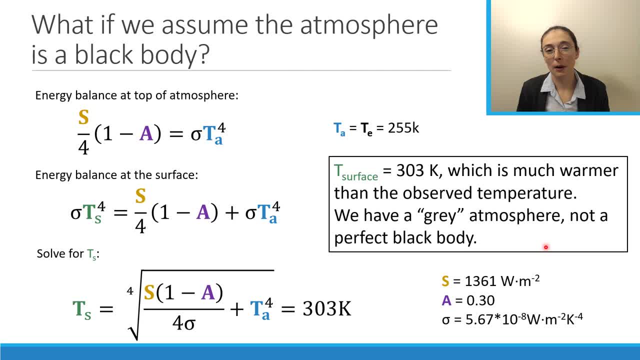 So what this implies is that we have a gray atmosphere, So that our atmosphere does not emit as a perfect black body, but it's a gray body, So it partially emits as a black body. OK, So let's talk about what a gray body is. 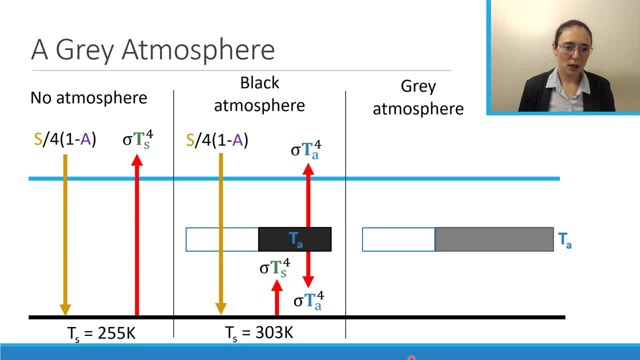 What a gray atmosphere would look like in our energy balance model. So, just as a reminder, our black atmosphere, our atmosphere which absorbs as a perfect black body, has incoming solar radiation which is absorbed by the surface and emitted as long wave flux. 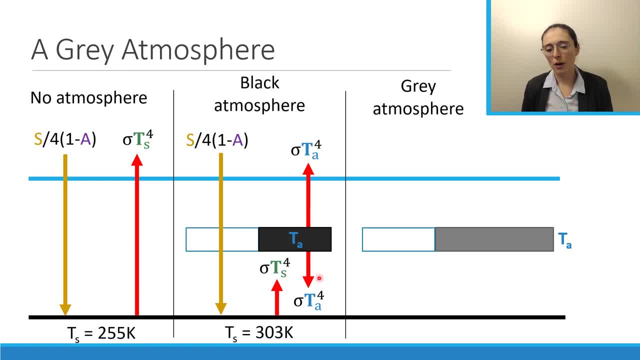 Now all of that long wave flux from the surface is absorbed by the atmosphere and re-emitted in both directions. Now, with a gray atmosphere, we still have our incoming solar radiation, which is incident upon the Earth's surface, And then we have outgoing light. 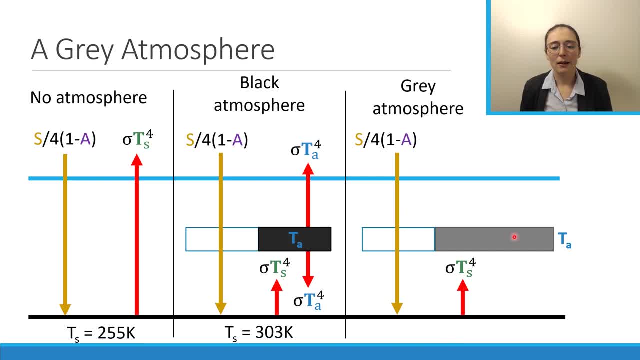 And then we have outgoing long wave flux from the surface And some of that light or radiation does get absorbed by the gray atmosphere and re-emitted. But some of the outgoing radiation flux from the surface is able to pass through the gray atmosphere and out into space.